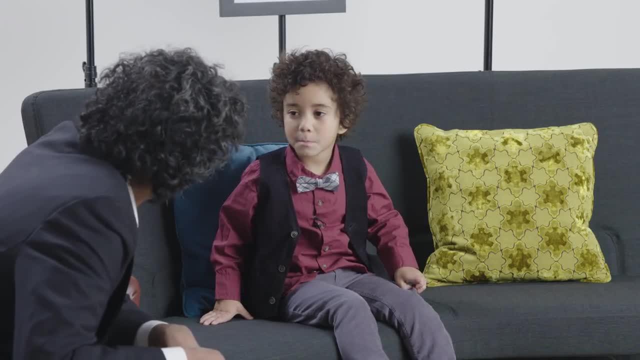 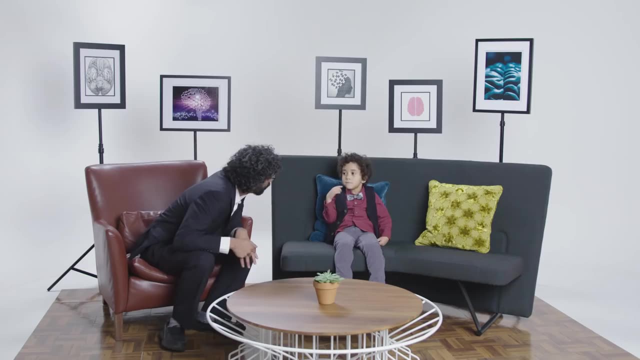 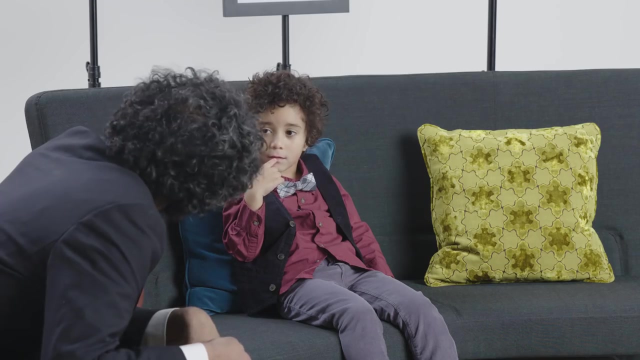 Something that helps you remember things Definitely. So what we're going to talk about this is something that people study in the brain called the connectome. Do you know that your body is made up of really tiny things called cells? Yes, I know that. Okay, well, there's more cells in your brain. 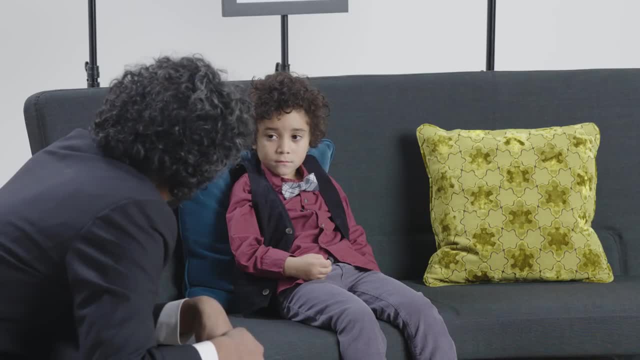 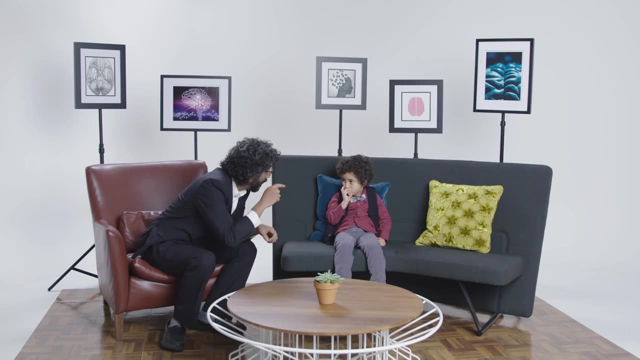 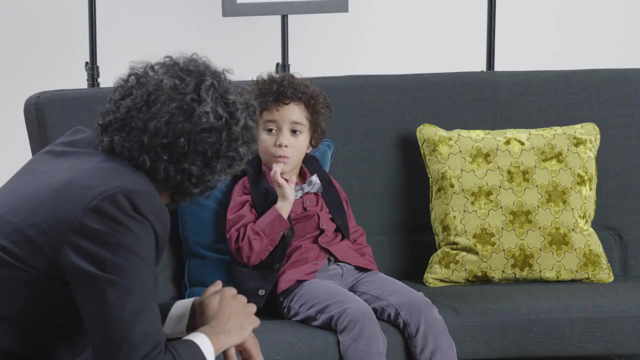 like way more cells than all the stars we can see, And so what the connectome is is we'd like to know where every cell in your brain is and how it talks to every other cell in your brain. That was awesome, Daniel, Thank you. 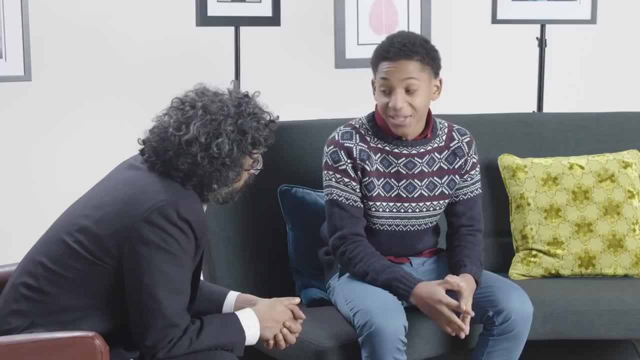 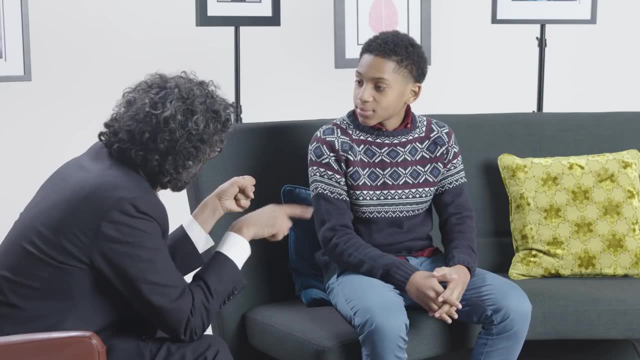 Connectome, Connect-ome. To be honest, I have no idea. That's good. That's a great place to start. There are cells in your brain. Those brain cells are connected by wires to each other. Electricity travels down those wires and communicates from one. 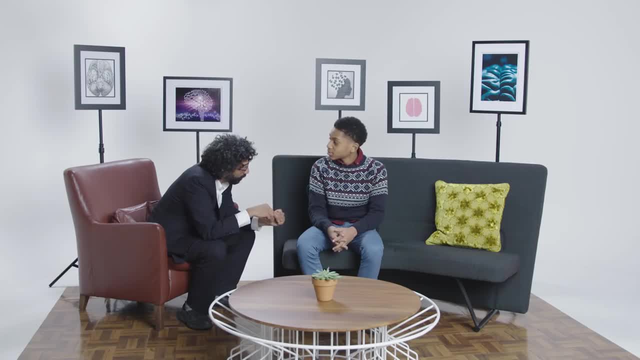 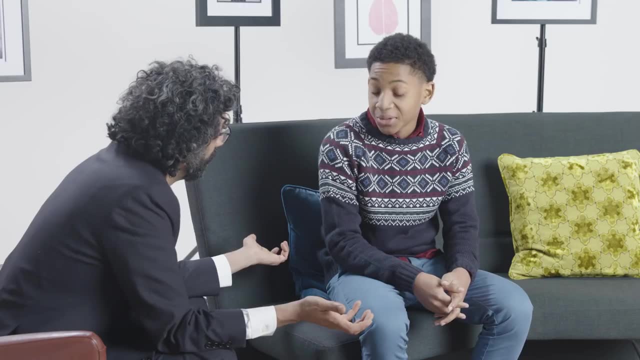 part of the brain, And when you do that it makes a connection to a certain part of the brain, So brain to the other part of the brain, and each of those brain cells makes you know a thousand connections, something like a hundred trillion connections in one. 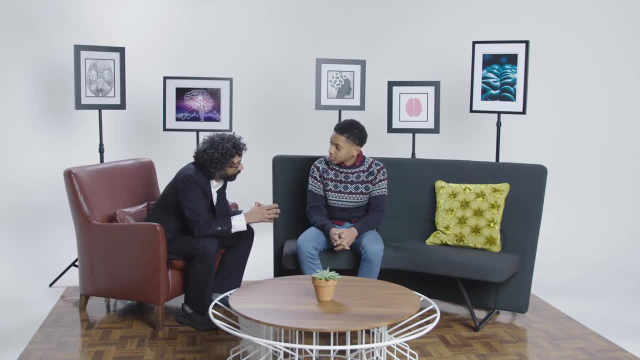 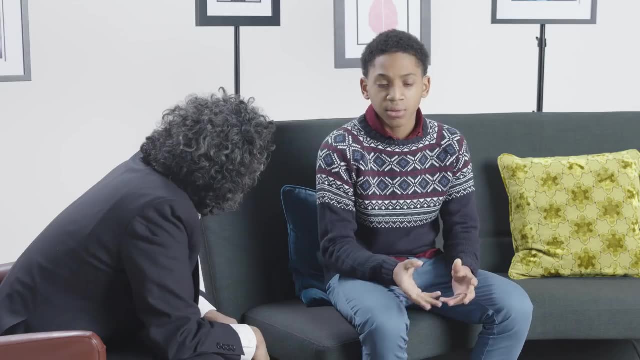 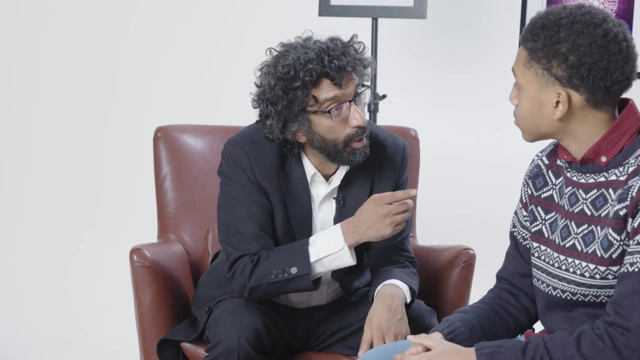 brain, in your brain. if could I take all of that information and put it inside a computer, would that computer then be you computers? they don't have feelings. they won't have feelings, and I think that's one thing that makes the human race wrong. I would say that that map also has your feelings in it, because here's why. 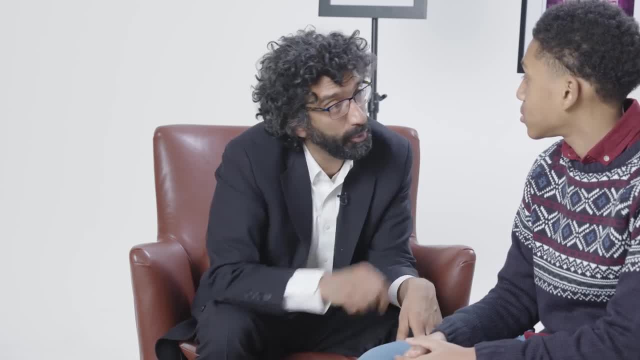 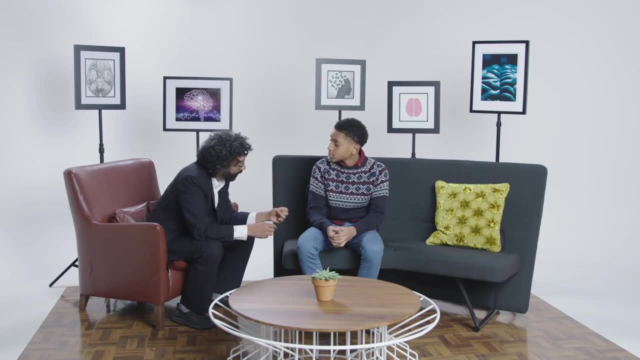 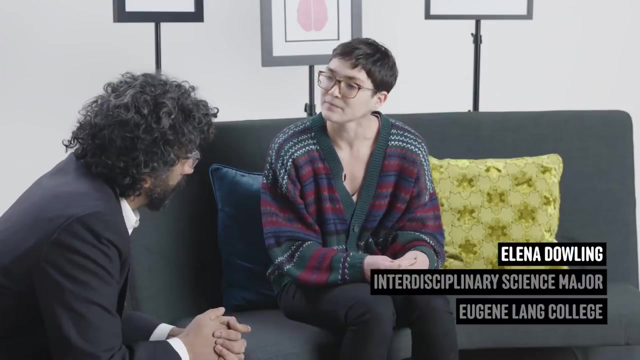 your feelings, most neuroscientists think come from your brain anyway and, amazingly, whether when you feel happy or sad or angry or scared, that's just brain cells communicating with each other. so I think today we're gonna talk about a connective. do you have you ever heard of that? I connect home. yeah, no, I don't. 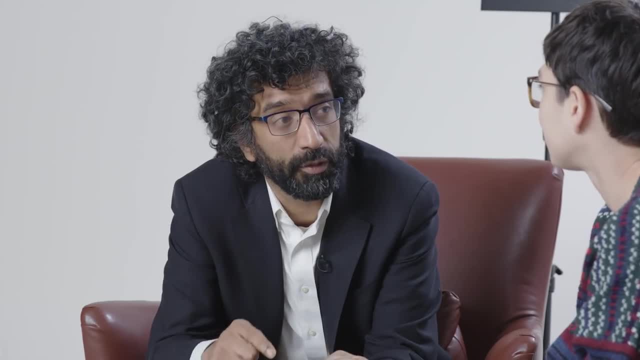 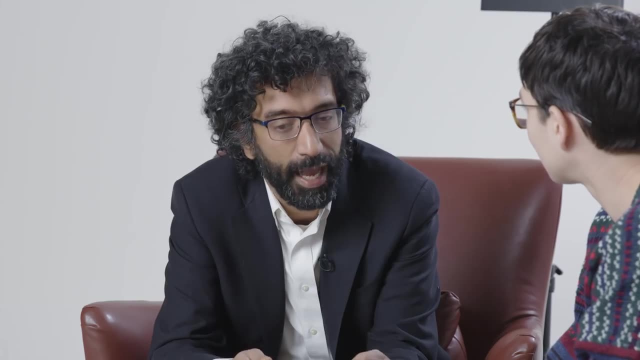 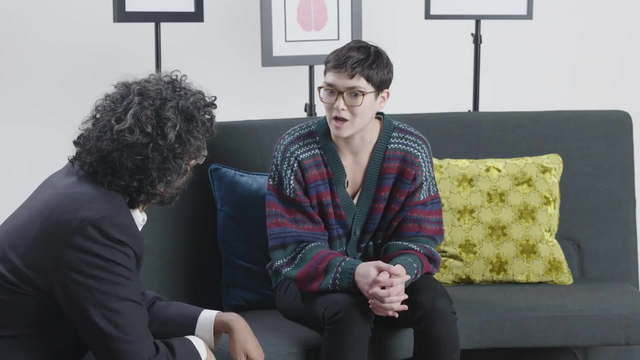 think so. it's a map of all the connections between every neuron in your brain, literally in a human brain, something like a map of the one quadrillion connections that a hundred billion neurons make with each other. is this like a map, where that's like an actual visual representation, like using microscopy or 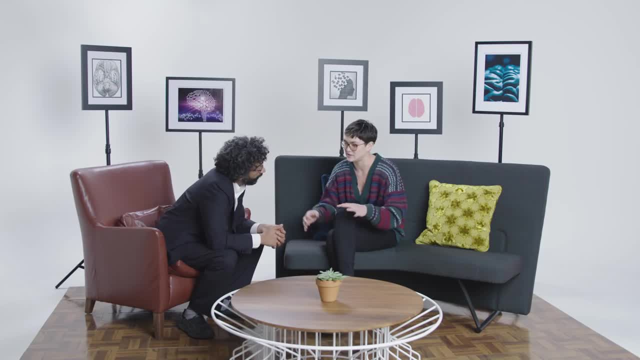 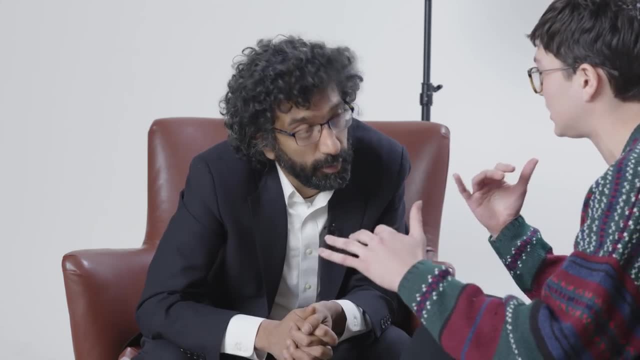 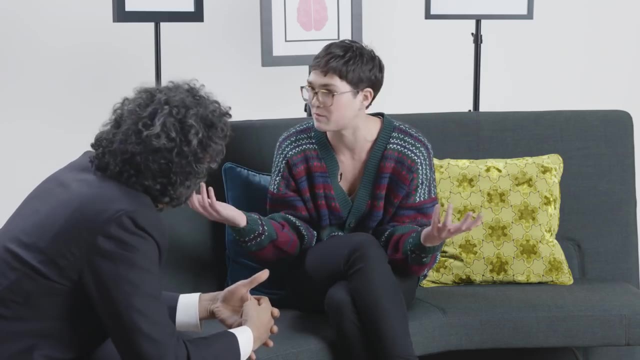 just data. Wow, I'm understanding more. so that it's these, these, the mapping of the nerve, the circuitry, the pathways between neurons that can lead to evidence of patterns in your brain that are common between different people. we have to use electron microscopic and then we've been developing a waste, sliced the brain into. really thin slices, use an electron microscope to take a picture of each slice and then use computers to put it all back. imagine that we could get the map of every connection right. and when you how neurons fire, do you think we could put that in a computer, that map, and then therefore that computer should be? 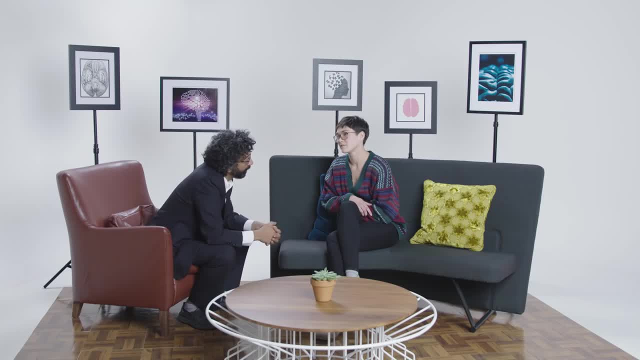 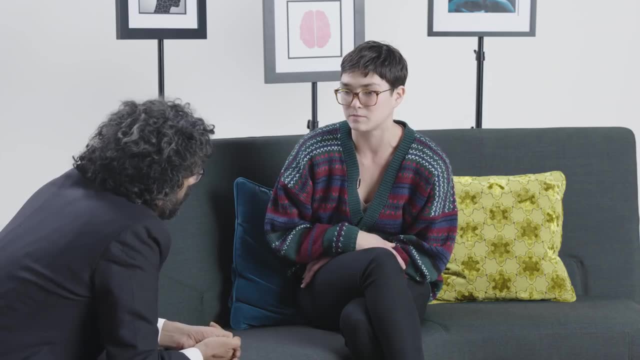 able to think, just like the brain that we extracted it from. well, the computer only communicates with itself in binary, so it only has two options. it can only ask itself yes or no questions, but a human brain has an infinity of directions that it can go. neurons are also. 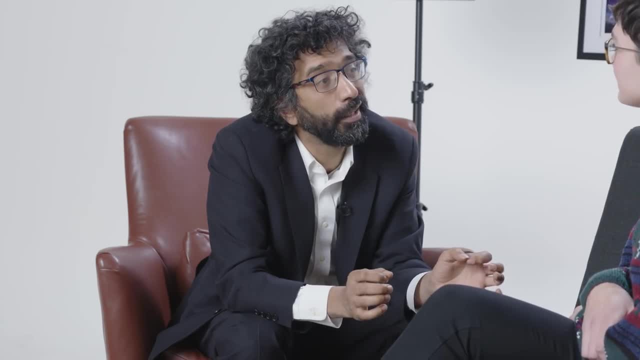 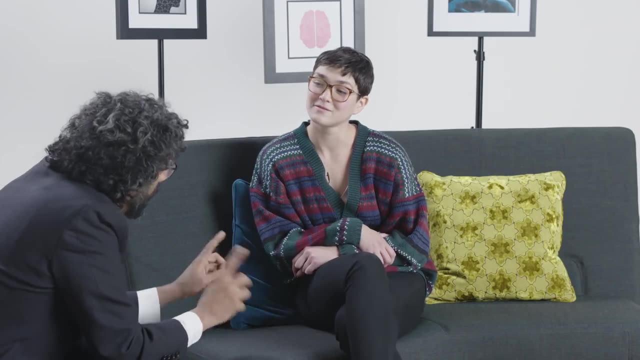 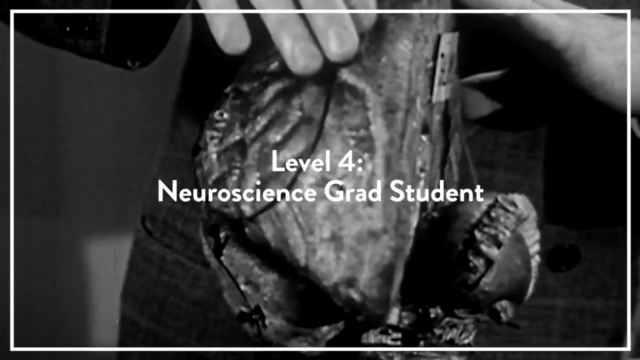 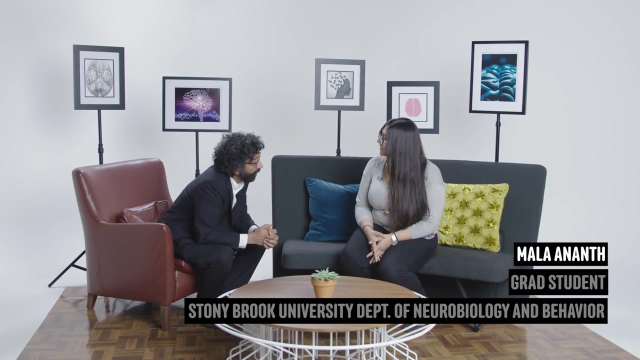 digital meaning a neuron either fires or it doesn't fire, so that's either one or a zero, and it's the combination of those ones or zeros that actually produce the 10 000 different answers that you say. it's a large-scale attempt to understand the wiring map of the brain. yeah, actually great, i think. 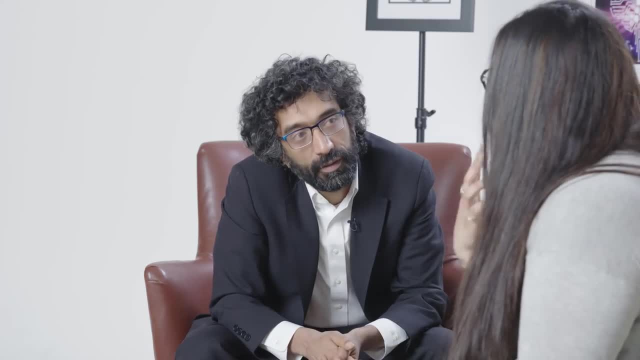 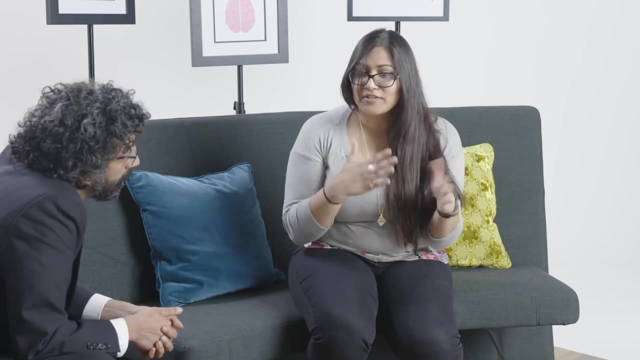 that it's definitely needed. understandably, understanding the anatomy of the brain is definitely important, but it doesn't necessarily tell us everything about the function, so there's some sort of temporal order from neuron to neuron and region to region that we may not be able to pick up. 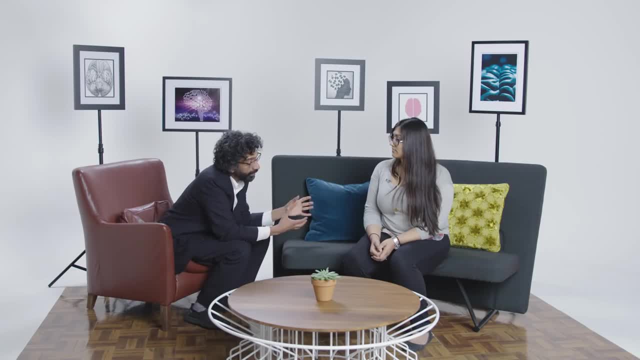 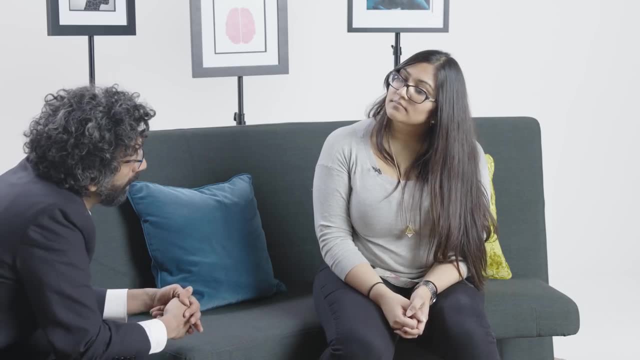 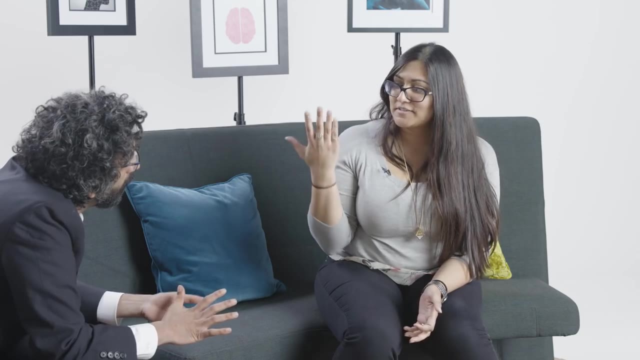 this is where it gets really crazy. could we simulate that map inside a computer, and would that computer then be thinking like that original brain for which we made the map? i mean, that's not. that's not the person. i mean, having a representation of someone's neural network is just that. it's just a representation of their neural network. i mean. 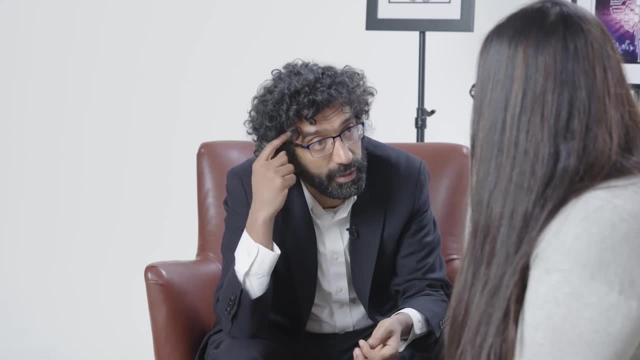 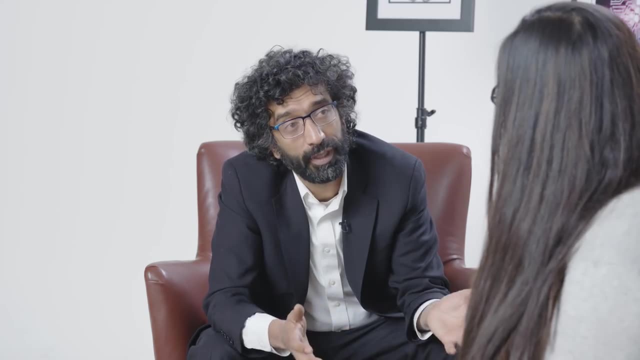 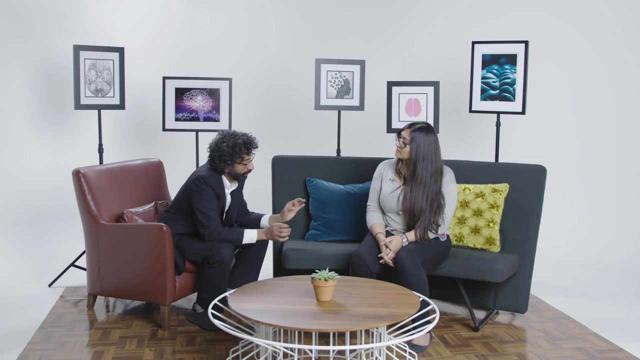 because there's more to the to you in here than just information passing between neurons. i'd like to think so. it would be like if you simulated a hurricane. imagine we can keep track of every variable of a hurricane- wind speed, every water molecule, etc. etc. temperature- and we put that. 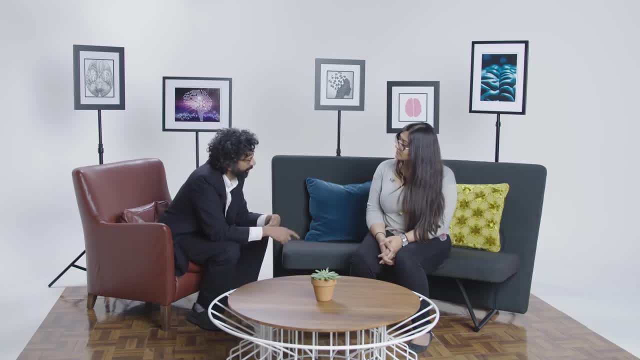 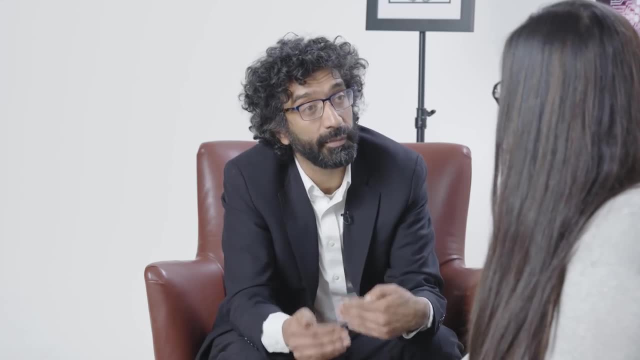 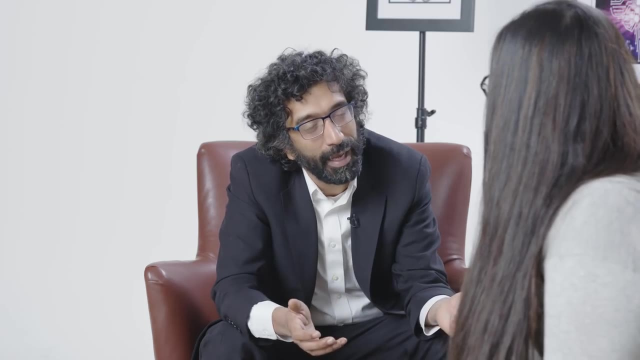 inside a super high-tech system, fast computer, and we simulated it right. i don't think anyone would think that the inside of the computer would get wet, uh, uh, even though we had simulated the hurricane perfectly. that wetness is consciousness is what we are. is it ethical to imagine mapping a male brain versus a female brain? 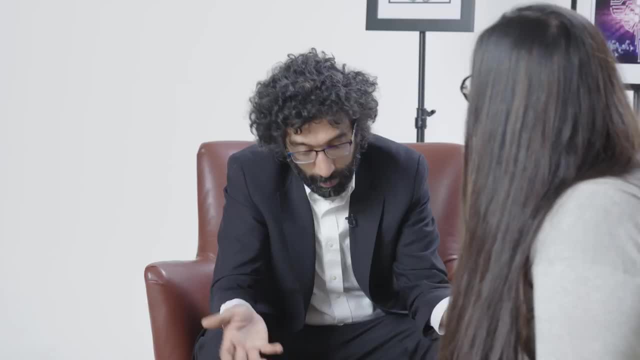 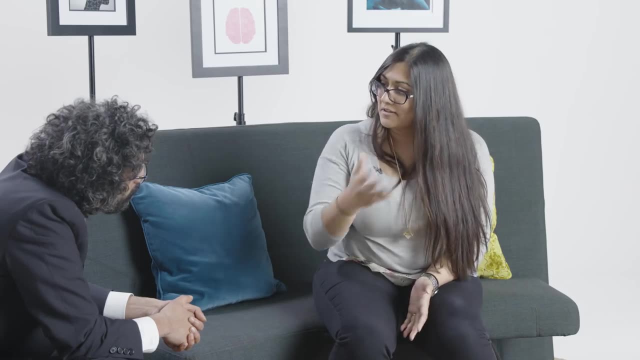 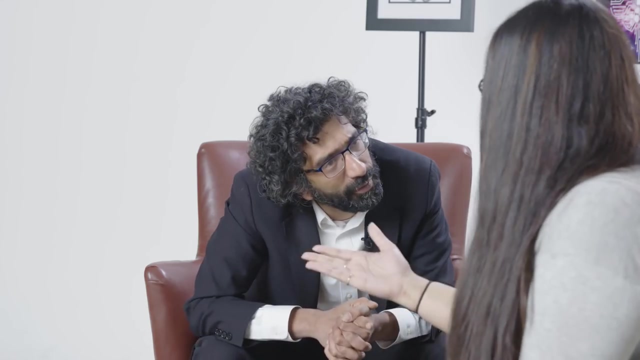 to look for differences between those, to explain alleged behavioral differences between them. every single person is different and so it should be okay to map every single person's brain. i mean, i understand that there are that. it's very sensitive. you know, what do you think is sensitive? mapping an indian brain versus a caucasian brain? or 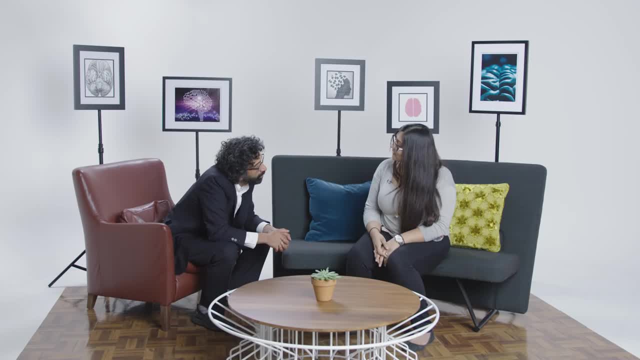 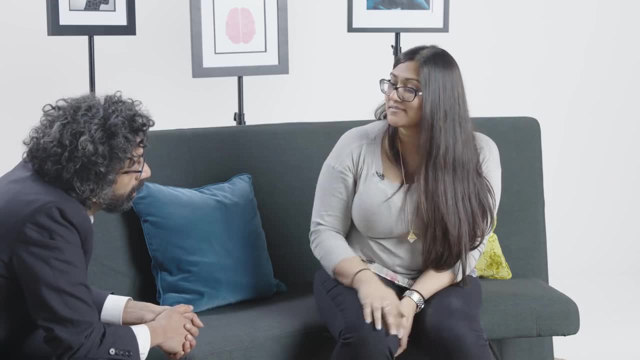 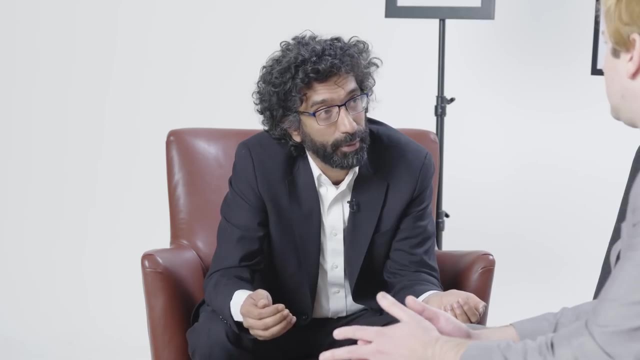 politically. i think that people may have some issue with mapping out what causes or what makes a difference between different types of people. maybe a wiring diagram is not sufficient to understand the brain, and it would be easy to think that that would be sufficient actually, if you limit the connectome to be. 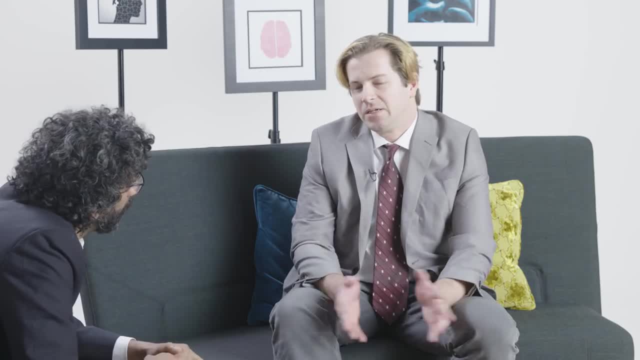 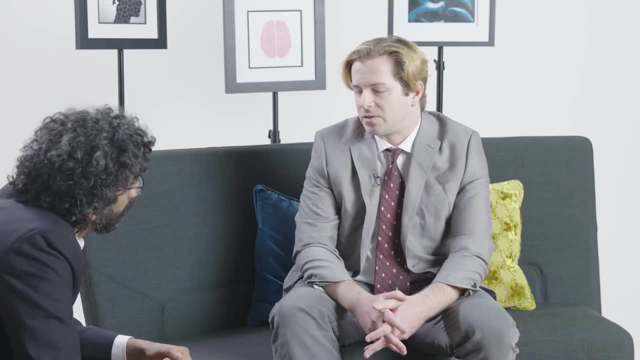 just the wiring diagram, without you know more information about, uh, myelination or glial cells, correct all types of environmental features that surround you, know the neurons and axons then then you have an incomplete picture, right? no doubt, sometimes when people get um, they worry about. 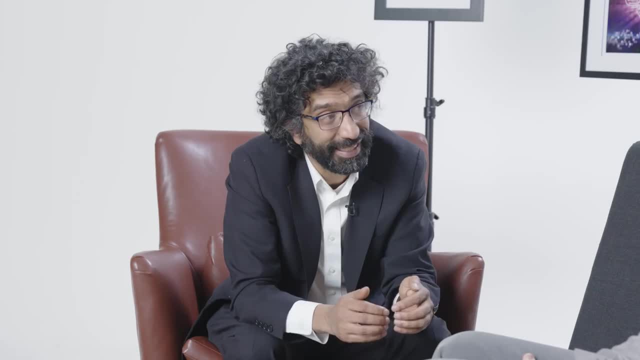 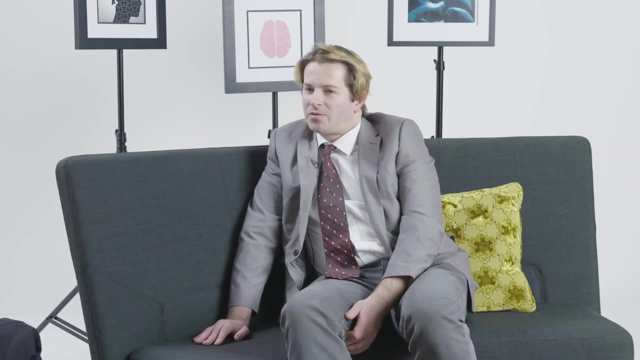 connectomics. i think what they're actually worrying about is that it's the end of the way that we used to do neuroscience. what do you think about memory? do you think that there's going to be a lot of? there's ways of resolving what the, the substrate of human memory is, you know? is it just ltp and ltd? 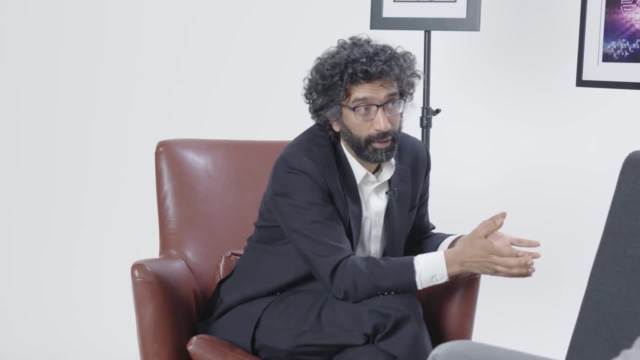 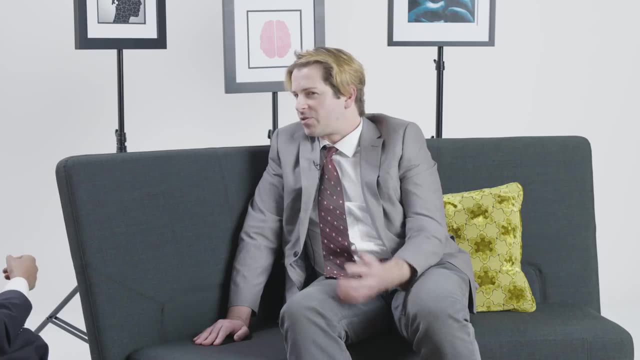 i'm not sure. if you had a connectome of a human brain, of an adult human, i would be able to read out memories from that. uh, uh. you don't think it's just the synaptic weights, like a, an artificial neural network gets trained to do particularly? it could absolutely be, but without knowing. 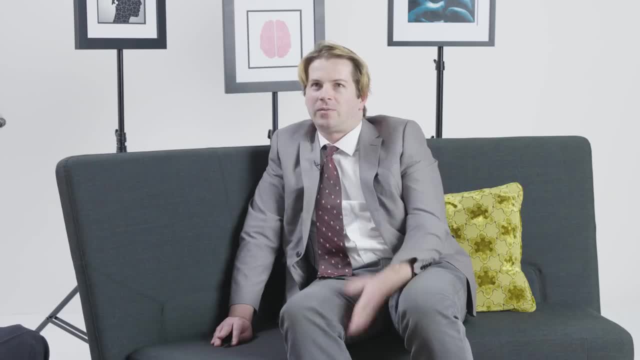 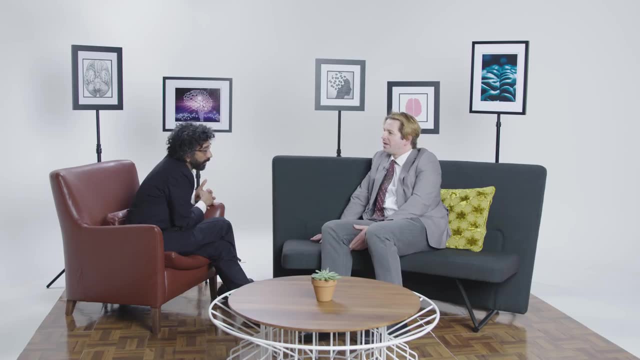 what the weights were before the memory was made. what if you, uh, had a violinist learn a piece of Bach music? and, yes, could you find those notes somewhere in their brain? yes, they didn't know before. yes, um, you know, i, i'm a musician, and i don't think it's possible. i think that there are.